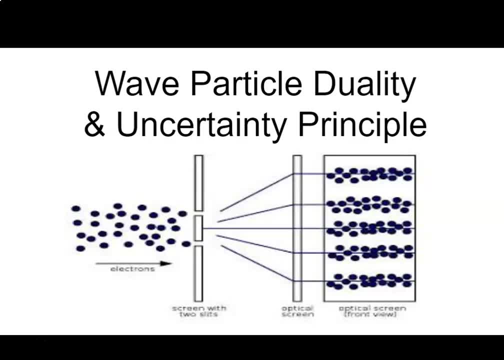 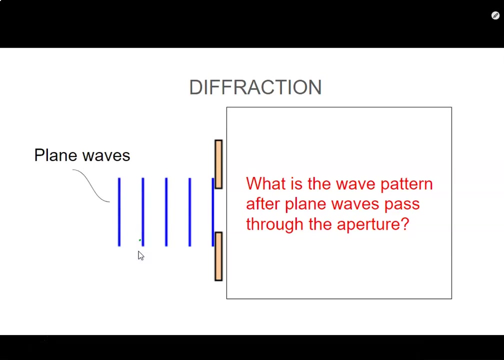 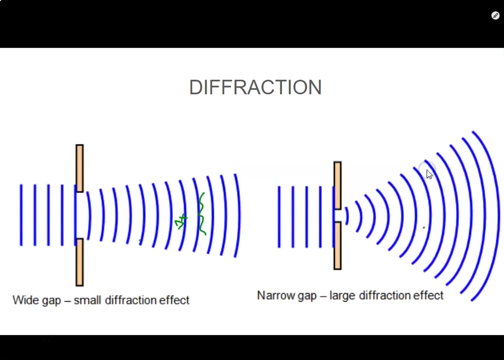 them. so. so so we already know the answer. this what we got: plane waves coming in. we have a slit of a particular width, and I'm going to call that X as opposed to D now, and we know that the what happens is, when we pass through, we're going to get a diffraction pattern. 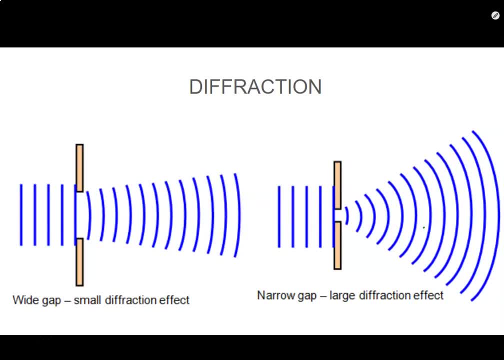 okay, now let's take a look at different diffraction patterns. if we have a wide gap, right, we're not going to get a whole lot of diffraction. in other words, that the gap is much larger than a wavelength, we don't get a lot. and if the gap is smaller or on the order of magnitude of the 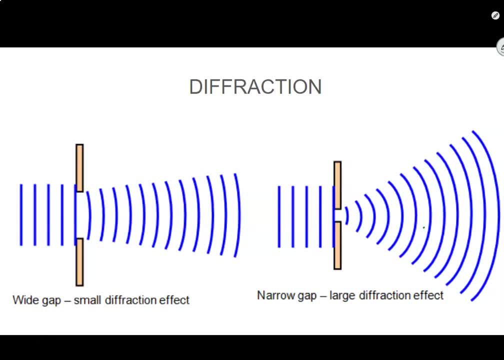 wavelength and you're going to get pronounced diffraction. so we can narrow. we can look at that progress of the waves this way and the spreading this way at some angle as essentially proxies for two fundamental measurements of that wave and or particle. Okay, and that's what we're really going. 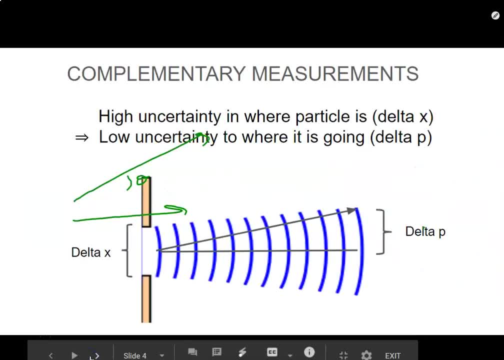 to focus on here, and this is the abstract part of it. All right, so I can unfortunately have to erase all those smart boards. So let's say that we have this gap width and we're going to quantify as delta x, where delta represents an uncertainty. In other words, if I want to know where is the 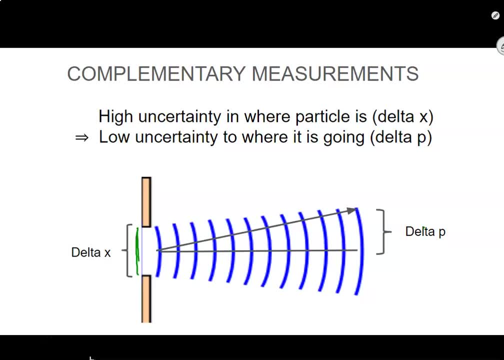 wave. it's somewhere between here and here. Okay, so there's some uncertainty in that delta x. Then we have another uncertainty that goes with it, and that is: where does the particle go? So, in other words, if the particle was here, we might expect it to go this way straight. 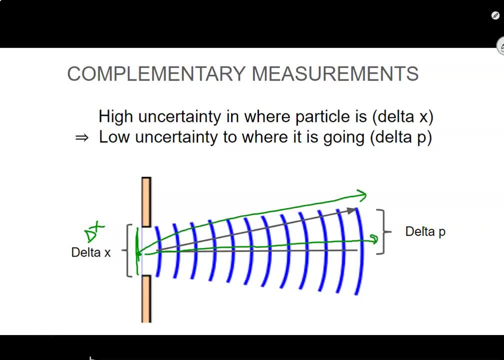 but because of diffraction, some of it's going to diffract that way or that way. so there's an uncertainty where it's going And how we measure the uncertainty where it's going is not so much velocity but rather momentum, Because momentum we want to. 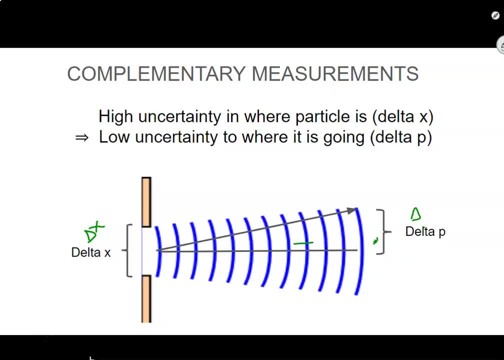 include the mass part, because if there's anything, axon that momentum is ultimately what matters as opposed to velocity. So let me reiterate, this is the key to understanding the uncertainty principle, at least from a classical standpoint. Again, we can say: where is the particle, Where is 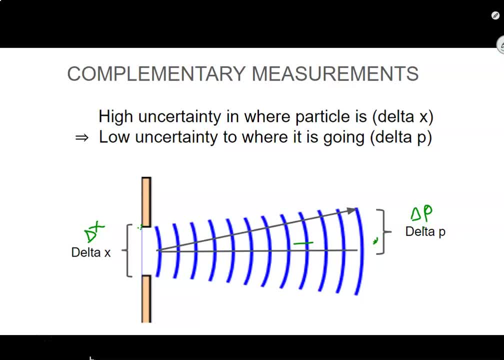 the particle, Depending on how small we make the gap. If we have a large gap, we really don't know where any particular part of the wave is. If we have a really small gap, then we can narrow it much smaller range And then we also can talk about where does the particle or the wave go once it. 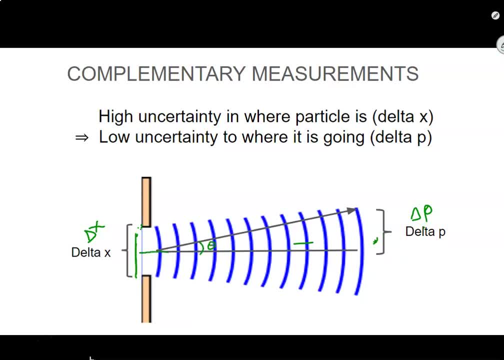 passes through the gap, and that's really the diffraction angle, which we're going to liken to the momentum Okay, where you are and where you're going, Okay. so in this particular example, we're going to be talking about the diffraction angle. 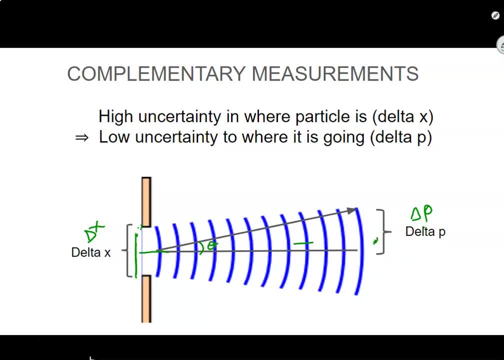 and, in this particular case, if we have a big gap, we have a high uncertainty in where the particle is. In other words, delta x is relatively large. However, we have a lower uncertainty, or a low uncertainty, in where it's going, which is basically a way of saying that the diffraction 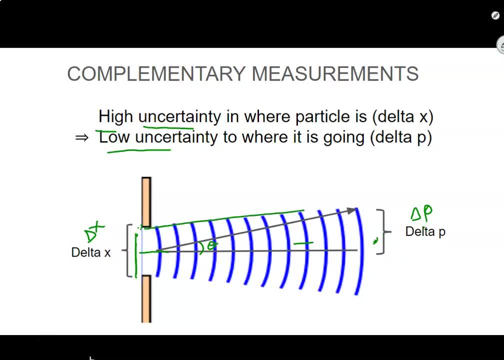 angle is fairly small, Okay, in other words, the range of possibilities is fairly small, because it's roughly the same size as the gap. So if we then change our gap, in other words, we make it smaller, we already know what's going to happen. 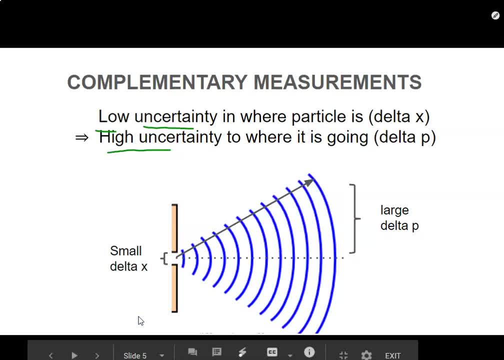 in terms of the diffraction right. So if I have a arbitrarily small gap, my uncertainty in x is pretty small, I'm pretty sure I know where it is. but I get a large diffraction so I get a large uncertainty in the momentum. So we get the reverse of what we saw. 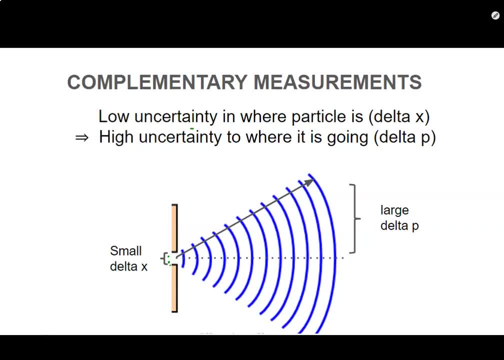 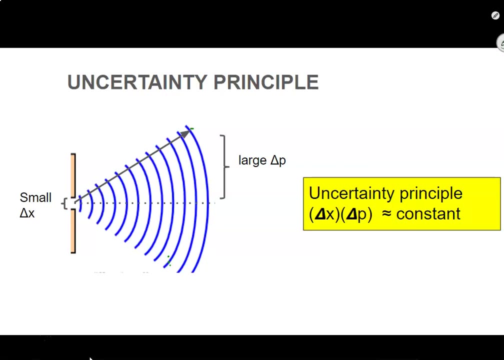 before. Here we have a low uncertainty where it is, but that corresponds to a high uncertainty where it's going. So what we're getting at is that ultimately- and this is fundamental to everything that is wavelength- is that you have a fundamental uncertainty in two measurements, And these: 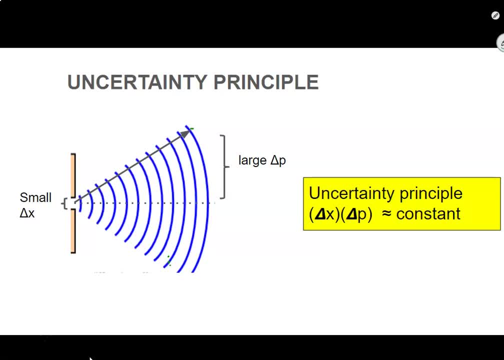 measurements are complementary. In this case, position and momentum are complementary, meaning that the less I know, the more I know of one. in other words, if this is small, the less I know of the other. Okay, so mathematically multiplying not the actual, but the actual, the actual, the 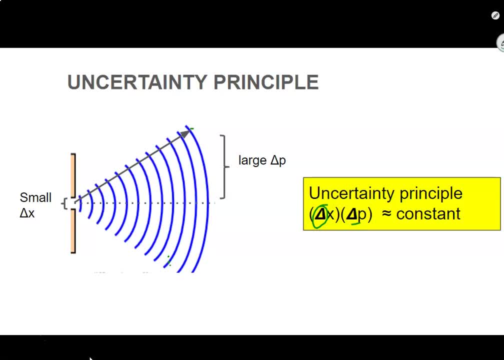 actual measurements, but the uncertainty in the measurements must be a constant value. So a small delta x- meaning I know where it is- means I have a large delta p means I'm not really sure where it's going, and vice versa. If I want to not know where it is, then I can know where. 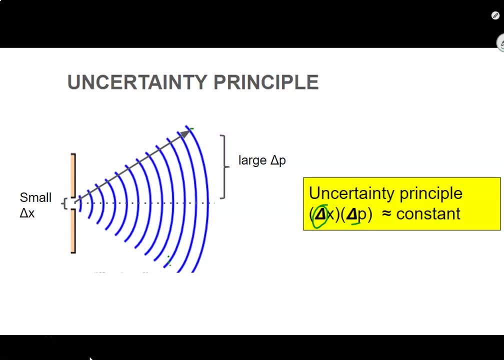 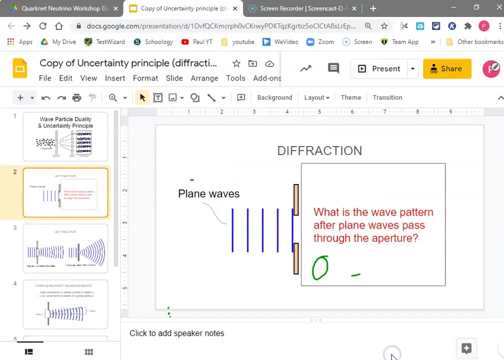 it's going, And that's ultimately what the uncertainty principle is about. It is a feature of all waves, and since particles have wave-like properties- electrons, protons- then this also holds for that, And that's certainly not obvious. So I am now going to turn to the note sheet and kind of 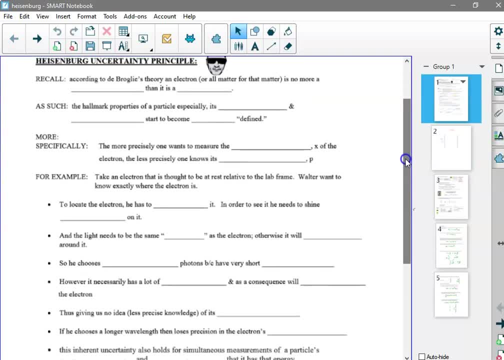 sum up this in a different way. Okay, so Now probably talked about this. According to de Broglie, there is no more a particle than it is a wave. It's one or the other, but it's not like nature prefers one over the. 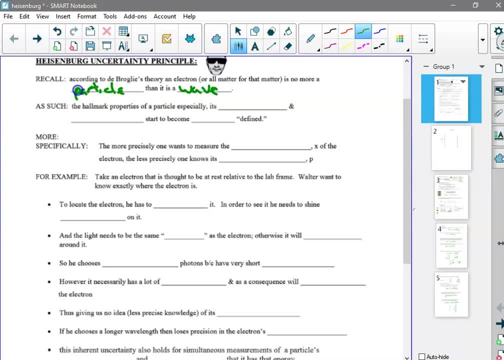 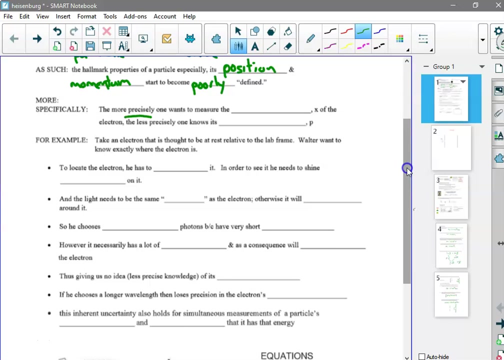 other, other and, as such, the hallmark properties of a particle, especially its position and its momentum, okay, start to become poorly defined, okay, so I'll go into that more. the upshot is more specifically, more precisely, okay, so that's precision, the uncertainty one wants to measure, the position, that's X. 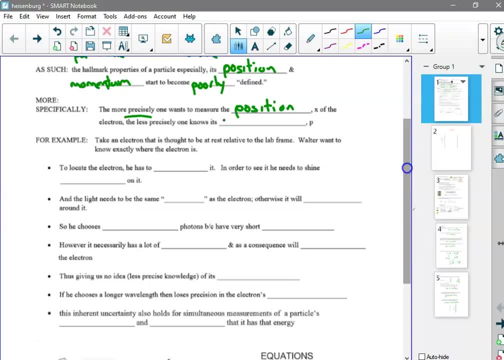 of the electron, the less precisely one knows where its momentum- and I was saying before, that's where it's going. so in a nutshell, basically measuring where it is- changes where it's going. okay, and that's not what classical physics tells us. the act of observing something does not affect what it's doing, but we're 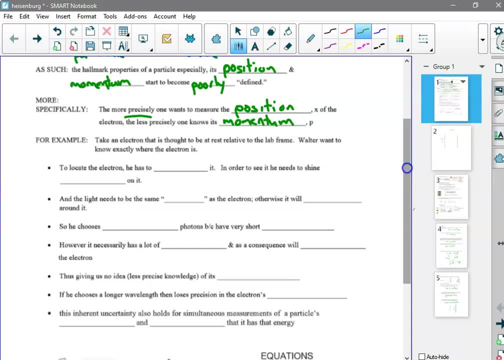 saying it literally does this. I gave you the wave analogy. now I'm going to give you another analogy based on the particle aspect of an electron. we can understand that, okay. so take an electron and let's say we've thought to be at rest relative to some lab presence, lab frame, and we 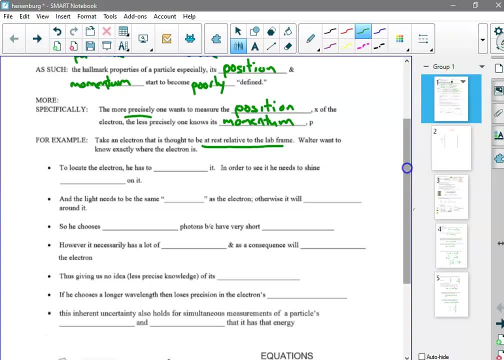 want to know exactly where it is okay. so we know there's an electron. we want to know where it is okay. so to locate where the electron is, you have to see it, not necessarily with the eye, but with some instrument. in order to see it we need to. 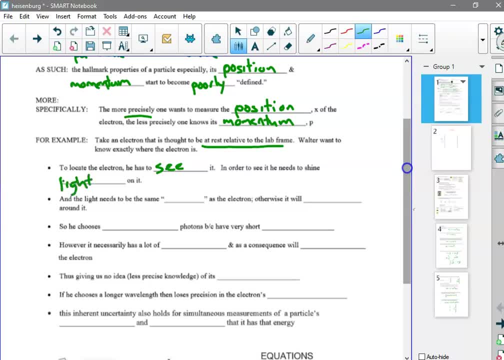 shine light on it, okay. and then light needs to be the same size as the electron, otherwise it will diffract right around it. so that's classical. we've talked about that before. if I want to look at an object and get a lot of detail from it, my wavelengths of 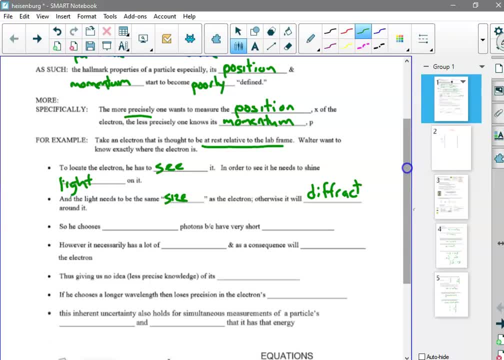 light have to be smaller than so what kind of wavelengths are we going to choose in order to see electrons? well, we're gonna go with this smallest possible, because electrons are really small. so let's go with gamma photons or X-rays, because you have a very short wavelength, okay, so 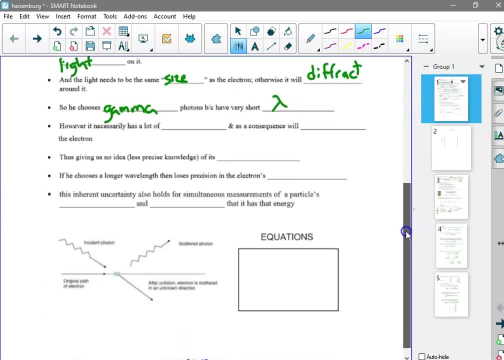 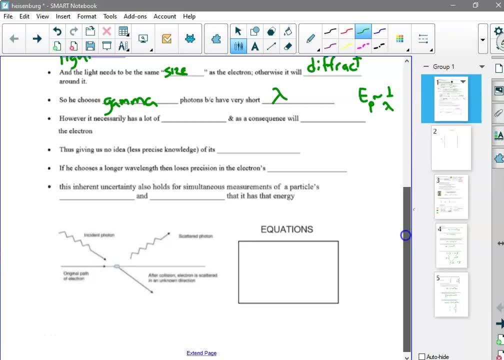 far, so good. however, now this is where Planck's law comes in. we know that energy of a photon is inversely proportional to the wavelengths, so we're gonna have a lot of energy, those photons of light, and a consequence, they will collide, or I should you know the collide with the electrons, or are they? yeah, I'm. 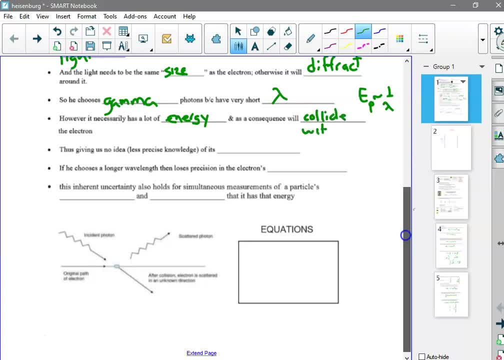 gonna put that in there, probably want a different term here- collide with the electron. okay, so by looking at the electron you are changing what it's doing, all right. in other words, if that photon collect- remember we had a stationary electron- we shine a gamma photon and do see it, but by virtue of shining that photon. 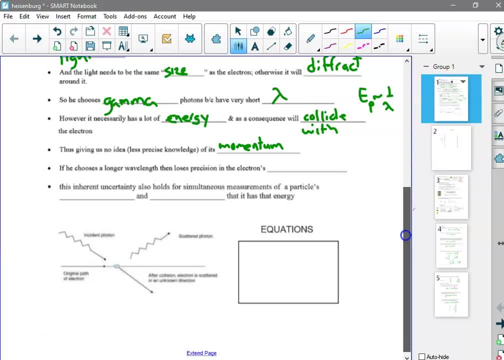 on it, we change the electron momentum, we lose information about where it's going. it's not obvious which way it's going to go, based on a collision. so if we don't want to affect the electron's momentum by observing it, we can choose a longer wavelength. in other words, it packs less. 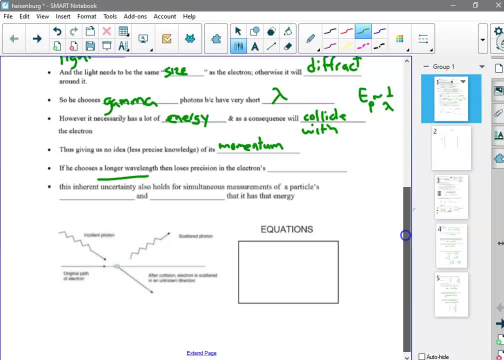 energy. however, if we choose a longer wavelength, then we lose precision, precision in the electron's position, because they're going to get more diffraction. there's really no way around it. so this uncertainty, this inherent uncertainty, also holds. oh, i'm sorry. so let's make sure we understand. 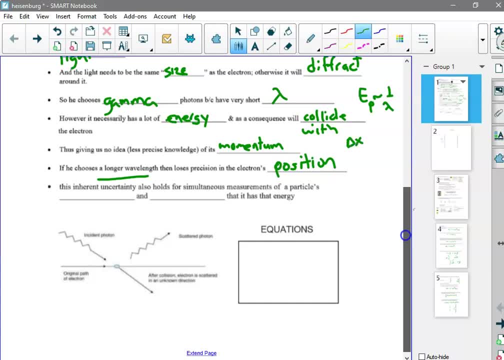 that if i want delta x to be tiny- in other words, i want to know exactly where it is- then I'm going to get a big delta P, because the act of looking at it is going to knock the electron off in an unpredictable way. If I want to have a small uncertainty of where, 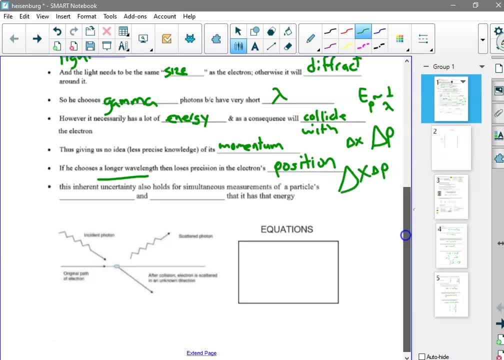 it's going, then I need a longer wavelength, which means I know where it is less precisely. So these two measurements are complementary. They have a fundamental limit to the precision I can know of one versus the other, And this is not an outcome of our instruments of technology. 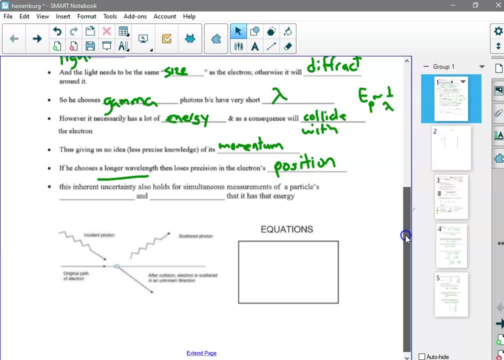 This is fundamental to nature, And it turns out there are other pairings of uncertainty measurements, And another one that we're going to talk about very briefly is there's a complementary between a particle's energy and time that it has that energy, So we can express the uncertainty. 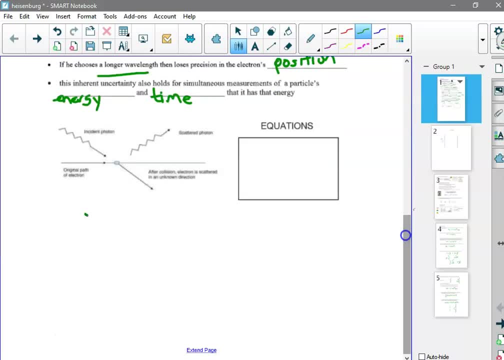 actually other ones as well, but we're not going to get into that. So here's a schematic of what I was talking about. Basically, we have a photon coming into electron Through the Compton effect. you've got a scattered photon and a scattered electron. So we can know where it was at the 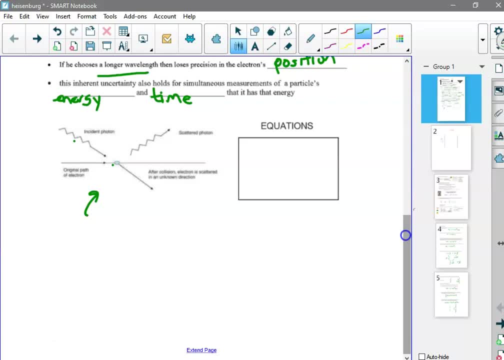 incident, but we changed where it was, so we don't know where it's going. Anyway. so the Heisenberg uncertainty principle can be written as: basically: delta X times delta P is greater than or equal to. So that's talking about the uncertainty. 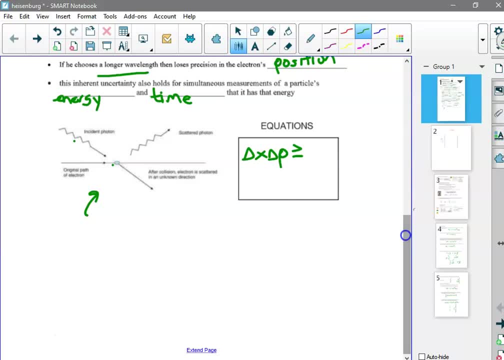 Okay, and it's a really, really small amount. As you imagine, it would be something to do with Planck's constant and it's H over 4 pi, So we're not going to derive what H over 4 pi comes from. 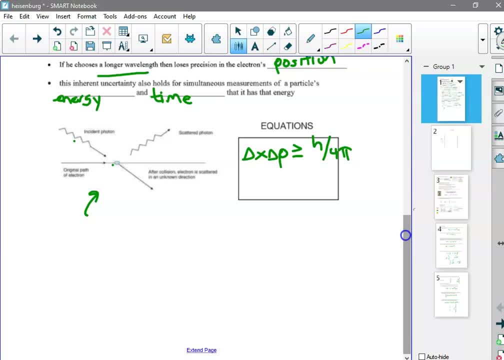 but that's in your IB part of your reference table under topic 12.. And then for the energy and the time, we have the same relationship. Okay, so again, this is not knowing. it's not saying we can't measure something's position exactly. We can, but by doing that we can't measure. 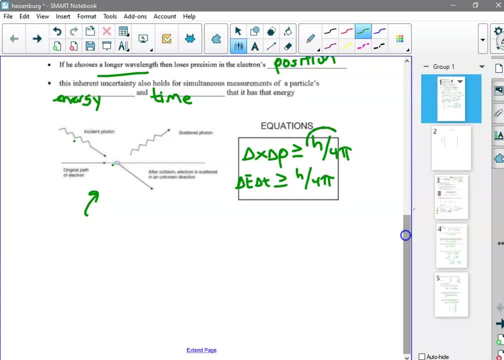 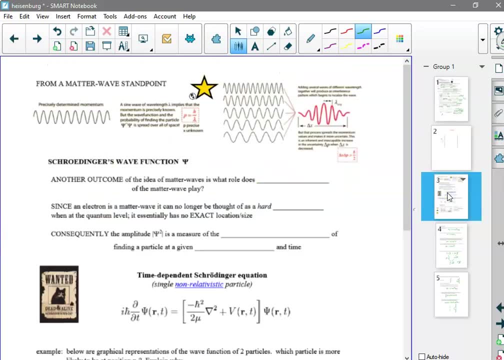 something's position exactly. We can, but by doing that, we can't measure something's position exactly, So we lose information about its momentum. And how much you lose is this, which doesn't seem like a lot, but at the quantum level it is fairly significant. Okay, now we can look at this another 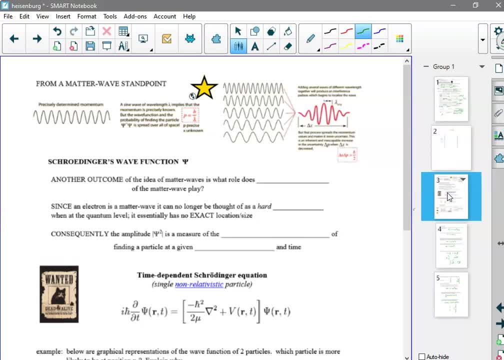 way, from a matter wave standpoint, and this is perhaps to me the most convincing. So let's say we have a wavelength or a wave, a matter wave, that has a very precise wavelength, Okay, and if it has a very precise wavelength, we can measure something's position exactly. So we can measure something's. 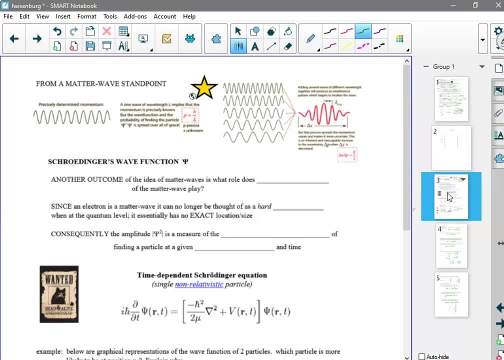 position exactly. So let's say we have a wavelength or a wave, a matter wave that has a very precise momentum. However, it's spread out over a large delta x, if you will. In other words, if I ask you, where is it? it's not really clear where it is. So, if you want to get a, if you want to understand, 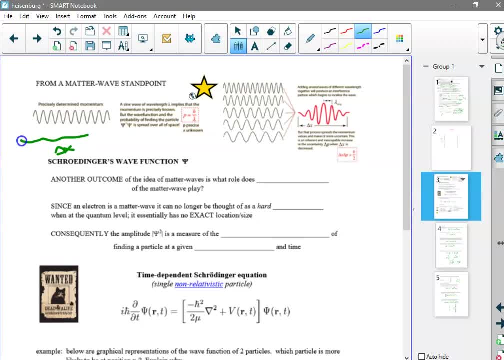 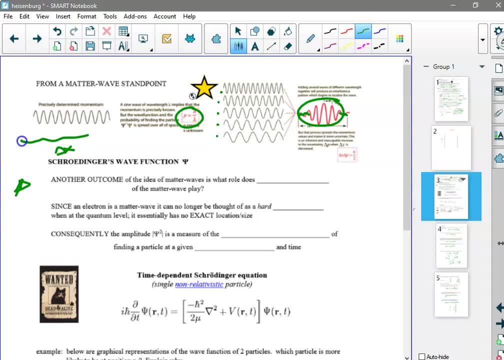 position: exactly So you can measure something's position- exactly So you can measure something's. 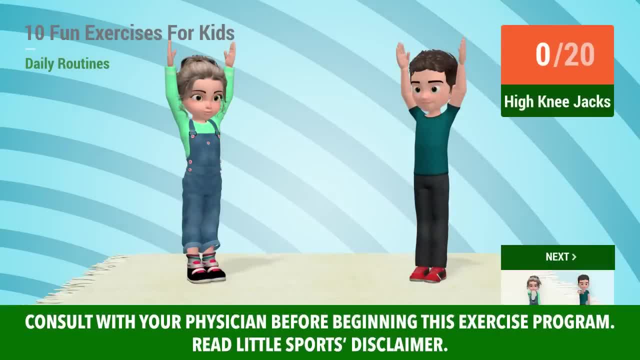 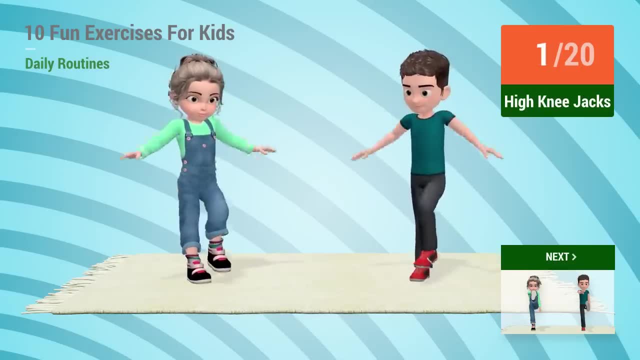 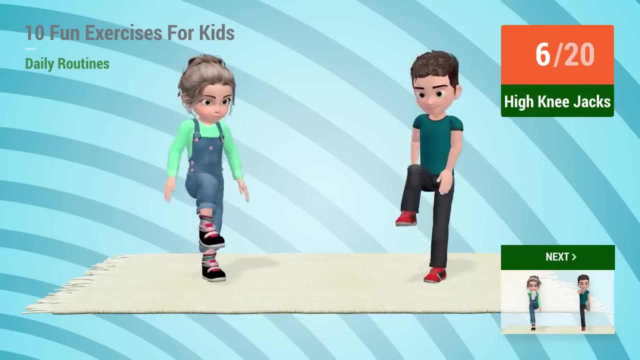 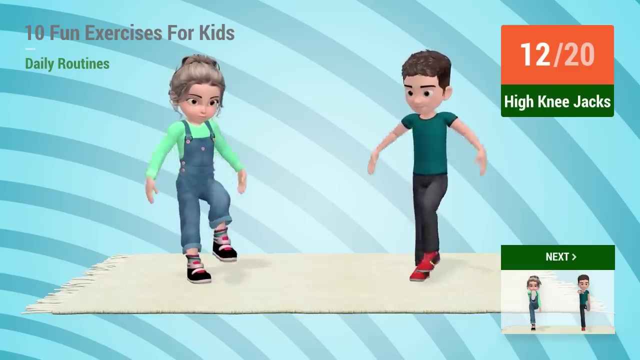 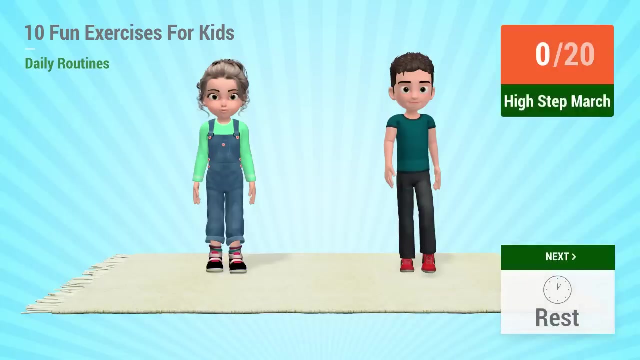 Up next high knee jacks in 5,, 4,, 3,, 2, 1, go. Up next high knee jacks in 5,, 4,, 3,, 2, 1, go. Step march in 5,, 4,, 3,, 2, 1, go.